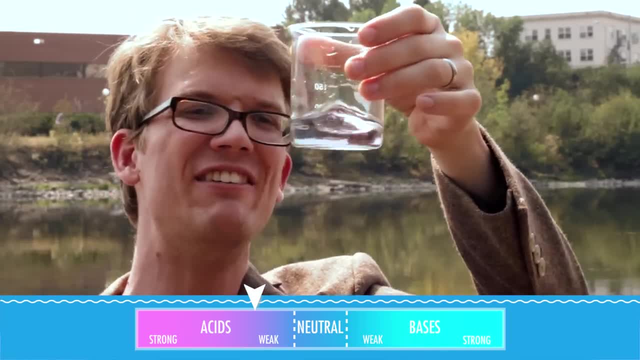 like five or six or seven drops. That was a lot more, And we're not even all the way there. Get – get a little bit more, Little bit more, Little bit more. Come on There, we go There There. Now it's acidic. 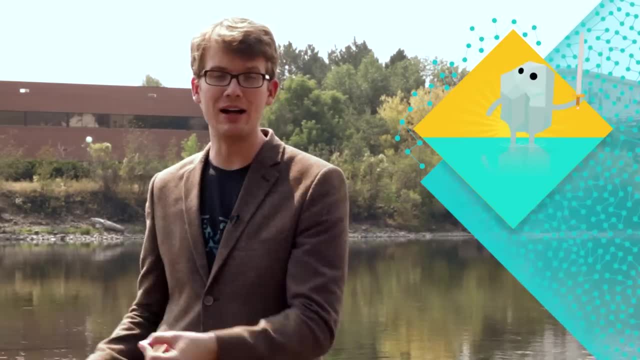 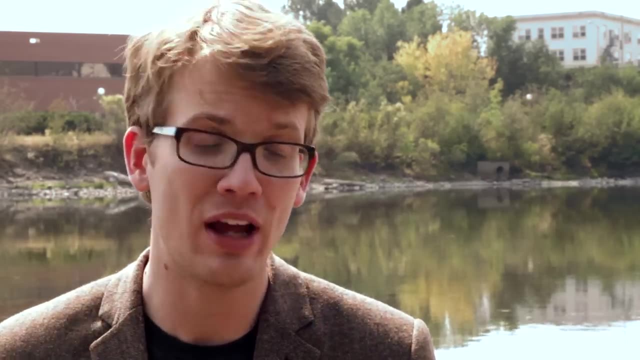 Why does this happen? It's because this river is protected by limestone, which is calcium carbonate that is present throughout the entire river system. Acid rain dissolves the calcium carbonate in the limestone. That carbonate washes into the river and acts as a natural buffer. A buffer solution resists changes to its pH when a strong acid or base 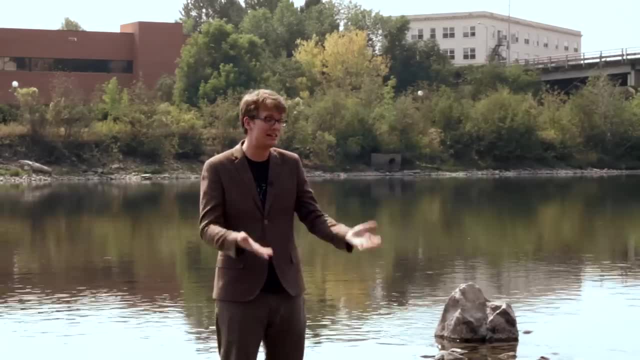 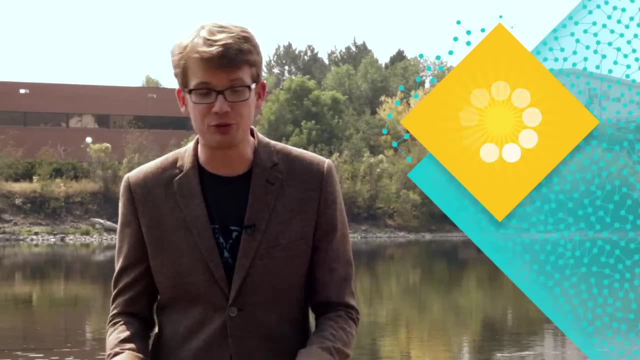 is added to it. So the Clark Forks Geochemistry explains why acid rain isn't as devastating here as it is in, say, the Adirondack Mountains of New York, where there is no limestone. Buffering is a big deal in chemistry. We buffer swimming pools to prevent the chemicals from 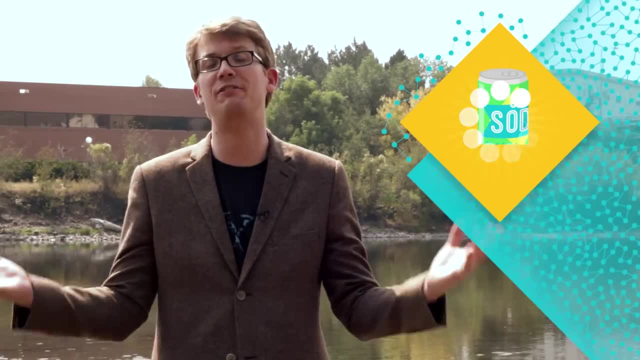 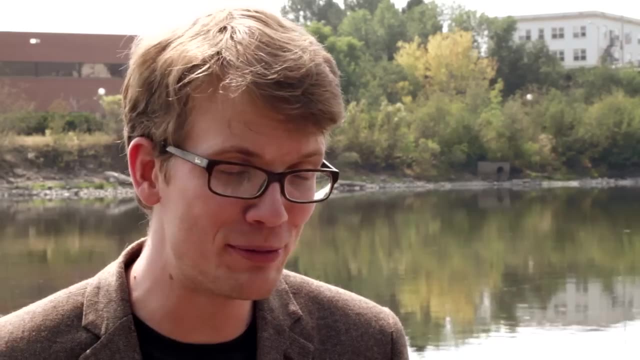 damaging our skin, and we buffer soda pop to prevent the acidic flavorings from damaging our teeth and tissues. We even have buffers in our blood to keep our internal pH constant and ourselves healthy. I think it's important to learn about something that powerful: How? 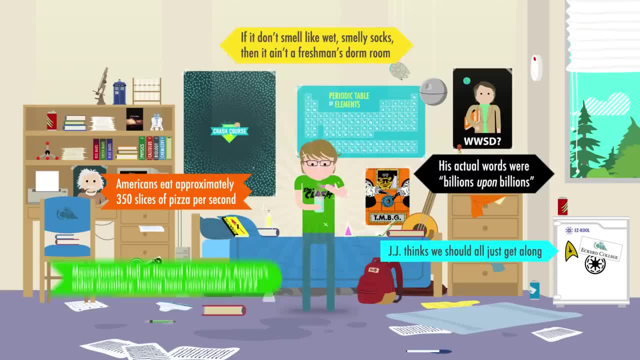 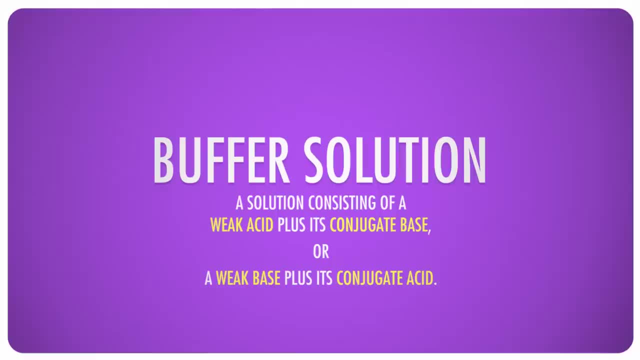 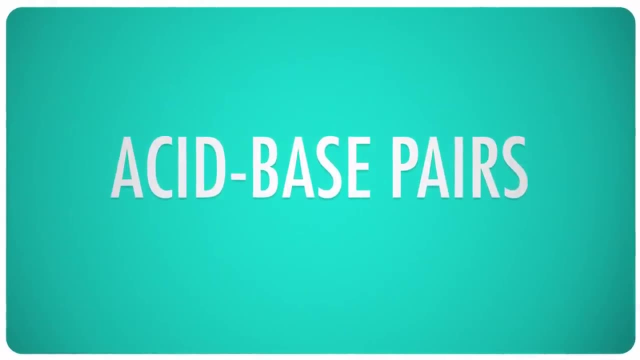 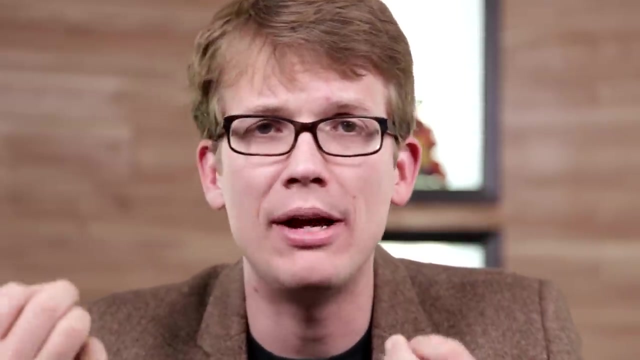 about you. A buffer solution is a mixture of a weak acid plus its conjugate base or a weak base plus its conjugate acid. These are called acid-base pairs. Weak in reference to acids and bases means that they only partially dissociate. It's actually their weakness that makes 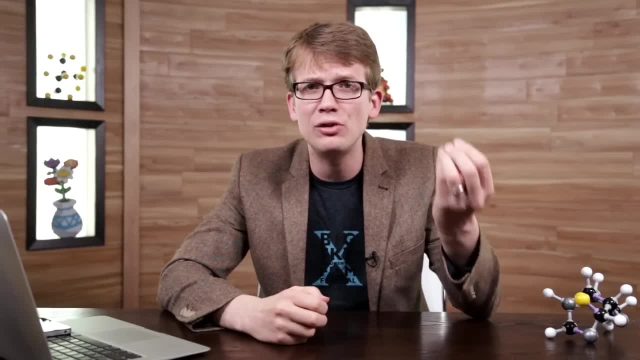 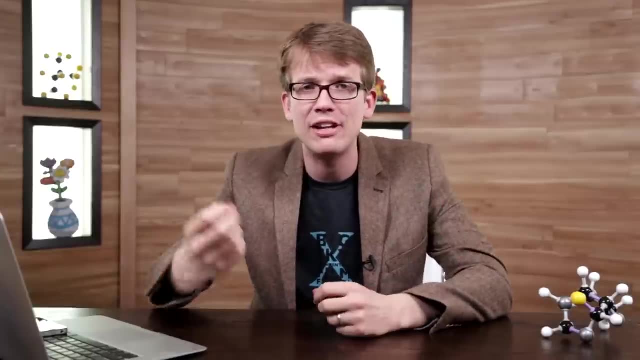 them great buffers, Since they don't fully dissociate in water. the undissociated buffer can act as either a source or a sink for protons, which helps neutralize a strong acid or base that's added to the solution. It's really all about equilibrium. For example, when a 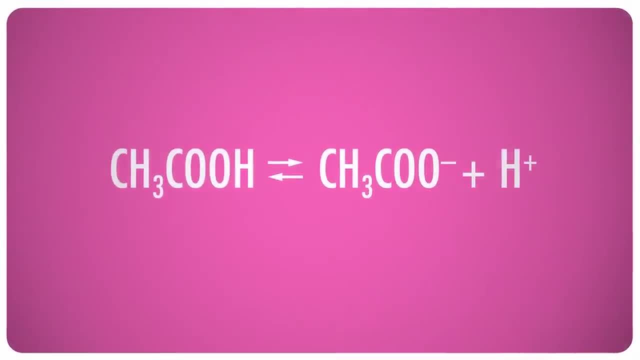 weak acid like acetaminophen is added to a solution, it's the same thing. It's. When acetic acid is added to water, a tiny fraction of it dissociates into its constituent ions, acetate and hydrogen ions, or protons. 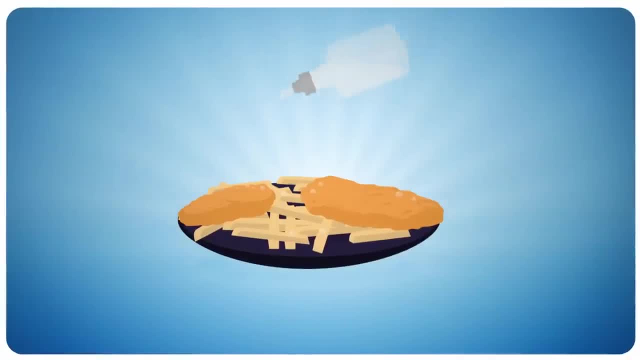 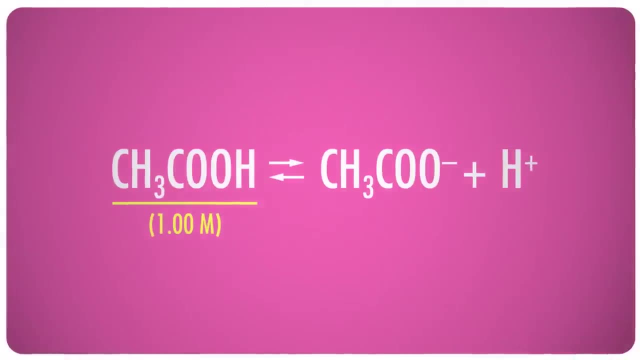 I was recently pouring a bunch of a solution like this all over my fish and chips. Vinegar is just a 5% solution of acetic acid, But the reaction is reversible as well, and that's where equilibrium comes in. Say, we have a 1 molar solution of acetic acid. 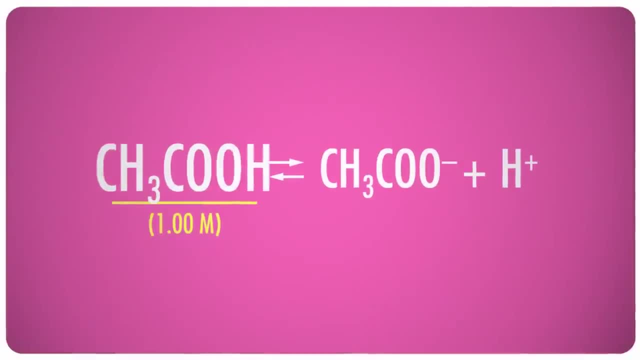 To make the solution a buffer, we need to increase the concentration of acetic acid's conjugate base, acetate, by adding sodium acetate to it. That would be a good way. Sodium acetate dissociates completely, thereby providing a ton of acetate ion. 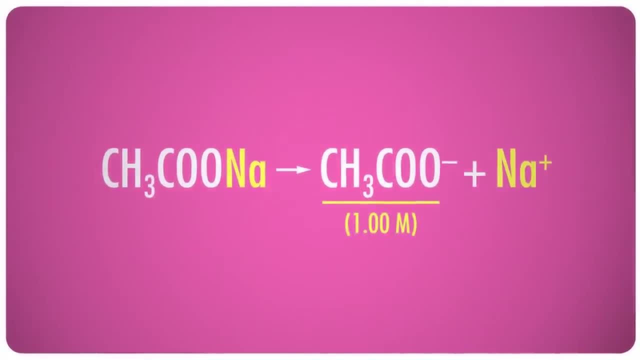 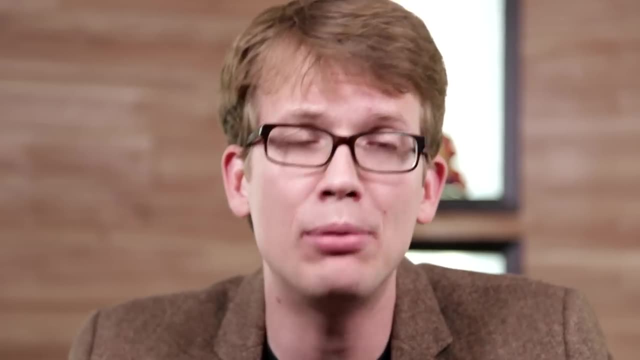 To see how this works in practice, let's add enough of that salt to make a 1 molar solution. We know how much acid and how much acetate we put in, but the important thing is the pH, And to determine that we have to know how many protons there are. 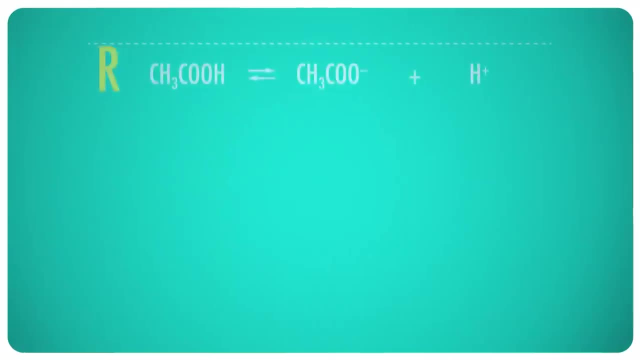 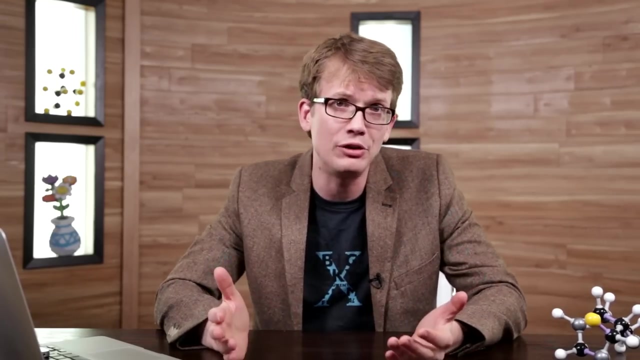 A rice table will help us keep track of everything. The reaction R we're interested in here, of course, is the dissociation of acetic acid. We can ignore the sodium from the sodium acetate, although it will stick around. 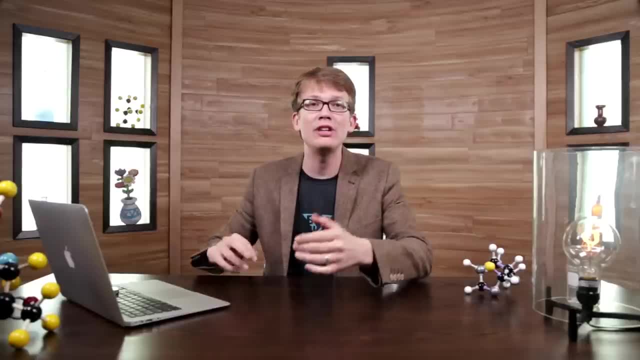 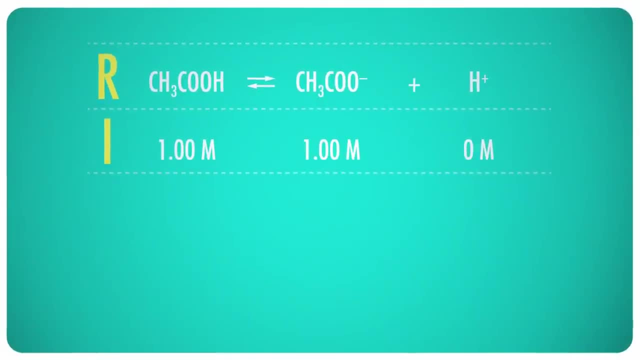 It's just a spectator ion that won't take part in any reaction. Our solution contains initial concentrations I of 1 molar acid and 1 molar acetate. We haven't formed any hydrogen ions yet, so that stays at zero for now. 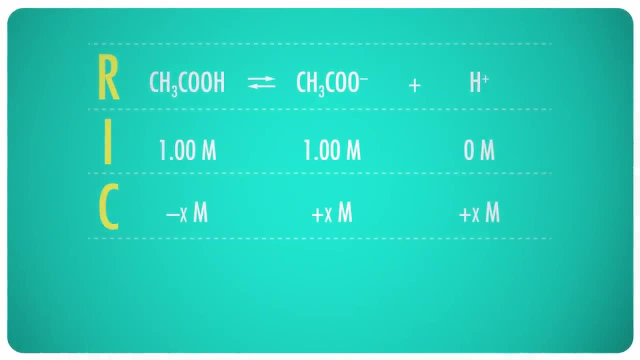 We don't know how much the concentrations will change C, so we call it X, The acid loses X and both ions gain X. So our concentrations at equilibrium E then are 1 minus X, 1 plus X and simply X in. 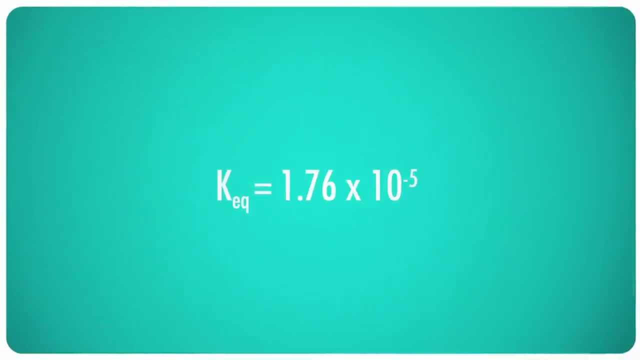 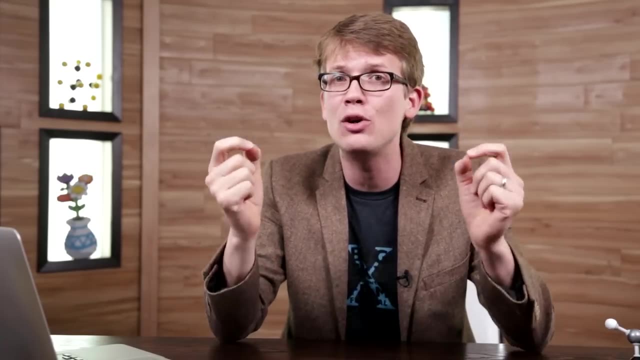 that order. Now to put the numbers into the equilibrium formula: 1.76 times 10 to the negative fifth. But when chemists work with dissociation equations for acids and bases, they give the Keq a special name: the acid or base dissociation constant. 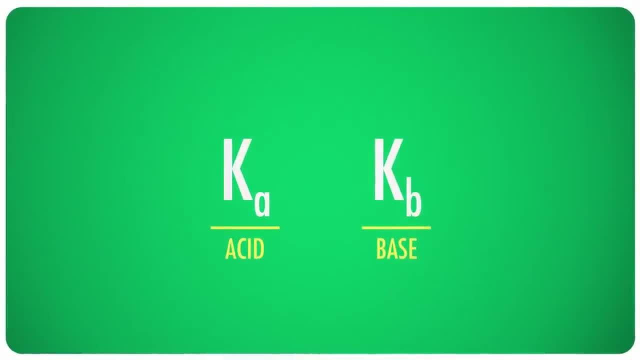 The symbol for this kind of equilibrium constant is Ka for an acid or Kb for a base. So use the equilibrium expression for acetic acid and put in the Ka and the equilibrium concentrations from the rice table. With a little simple algebra it simplifies. 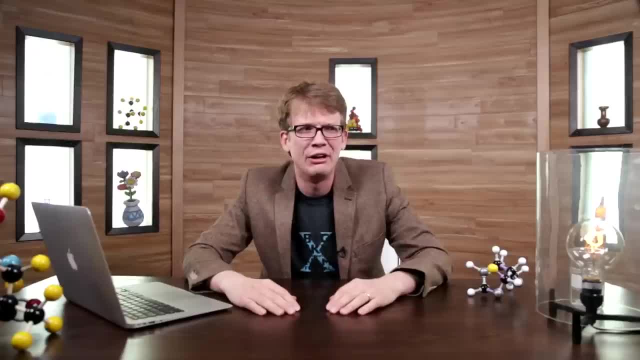 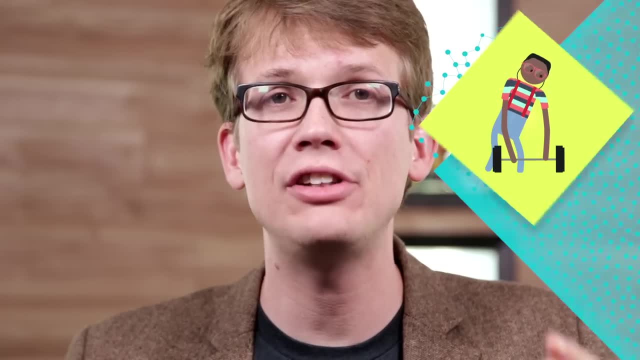 That doesn't look simplif- I guess you could call that simplifying, but that's like quadratic. I don't want to do that. So here's a little trick to make this a lot easier. See, acetic acid is a really weak acid, so only a tiny fraction of it dissociates, which 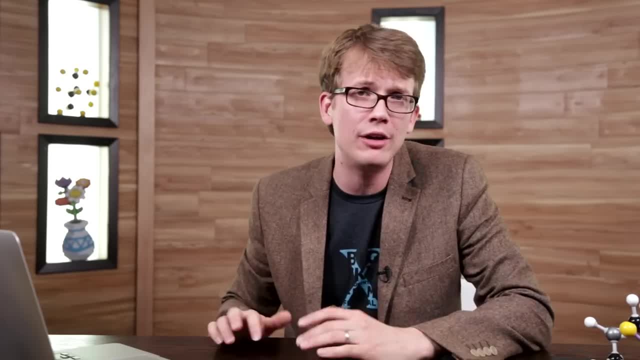 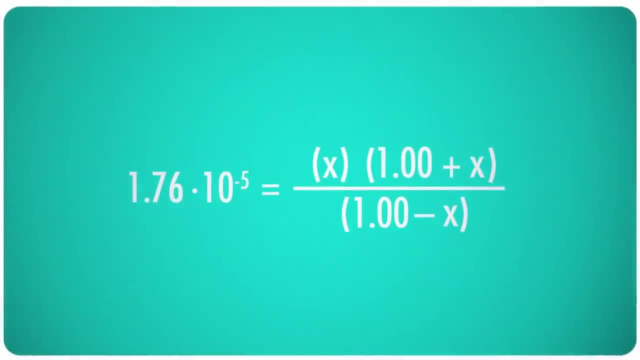 means that X is super small. If it's so small that after rounding for significant digits it doesn't change our answer at all, then why not just drop it, Now that first X for the hydrogen ion has more effect because it's multiplied, but the 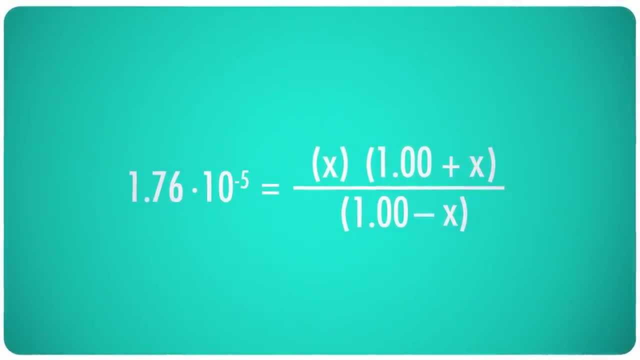 other two. Let's just forget they're there and see what happens. If we go back to where we plugged in all the numbers and simply drop the two Xs that are being added and subtracted, the rest of the problem cancels out, leaving X. 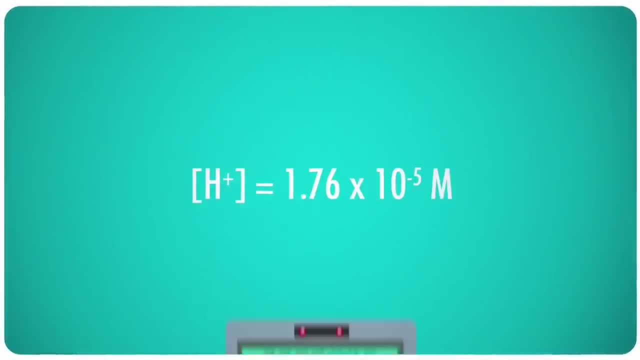 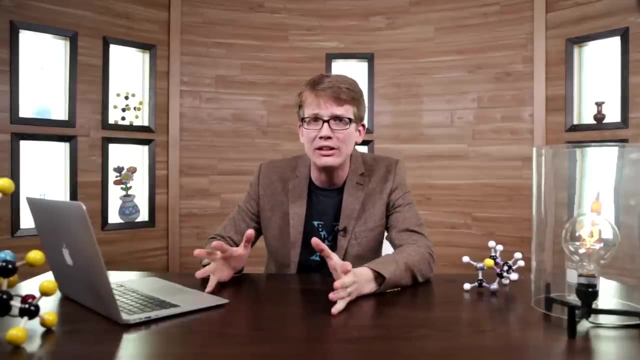 The rest is a breeze. with a couple of taps of the calculator, we find that the pH is 4.754.. But here's the big question: What if we try to push the pH out of whack? The whole point of a buffer is to resist that right. 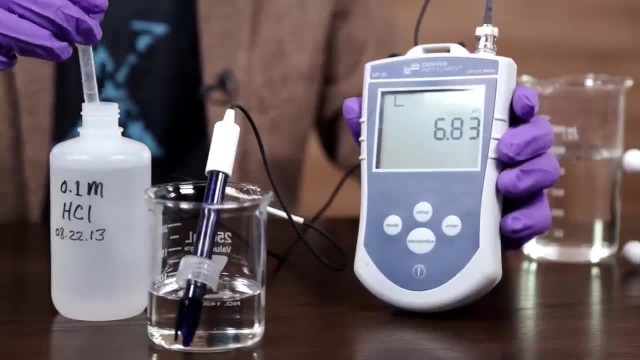 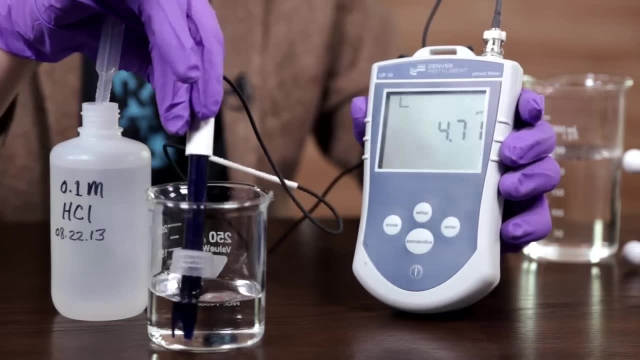 If I add a strong acid like, say, hydrochloric acid, at a concentration of like 0.1 mole per liter to distilled water, the pH will change very quickly to like very fast dropping. yes, Now we're at like three pH of three. 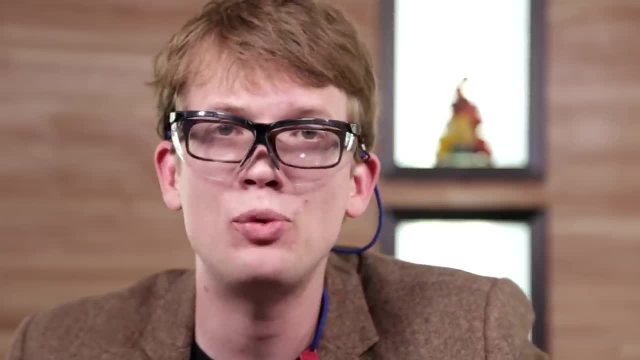 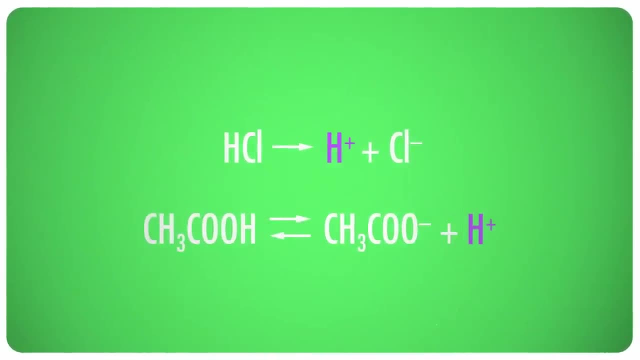 Not a healthy environment for most orchids. Well, let's think about what would happen to the pH with a buffer in place. Even though HCl dissociates completely in water, releasing tons of hydrogen ions, when it's added to a solution that's buffered with acetate, the excess hydrogen ions join. 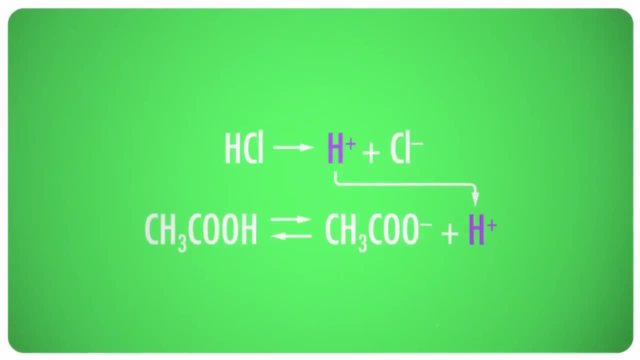 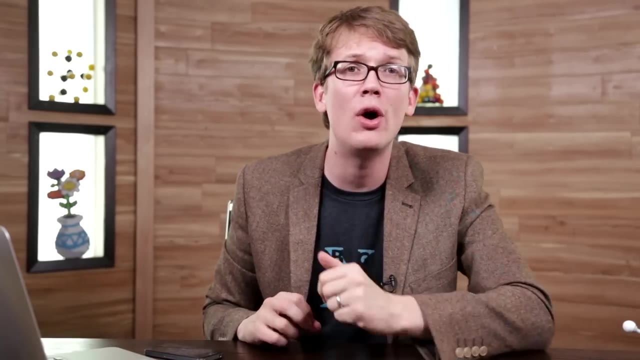 with the acetate ions to form acetic acid. Thus that strong acid can't affect the pH much. because the hydrogen ions are used up To neutralize 0.01 molar HCl or more specifically 0.01 molar H+, the acetate concentration must 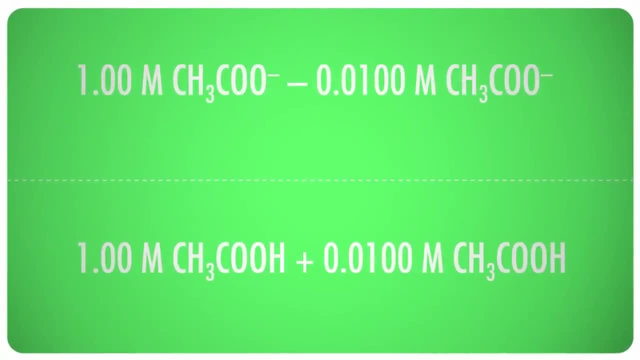 decrease by 0.01 moles per liter, simultaneously increasing the pH of the hydrogen ion. That's what we're looking for. We're basically increasing the acetic acid concentration by 0.01 moles per liter. That leaves us with 0.99 molar acetate and 1.01 molar acetic acid. 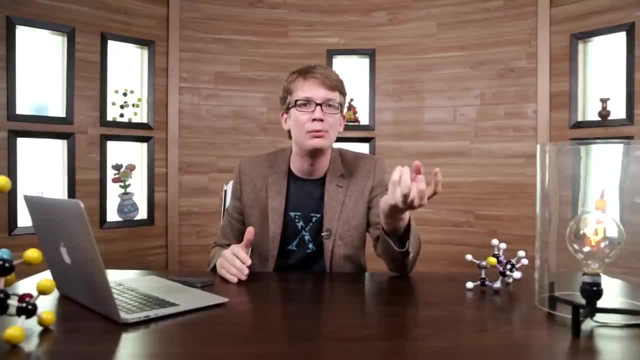 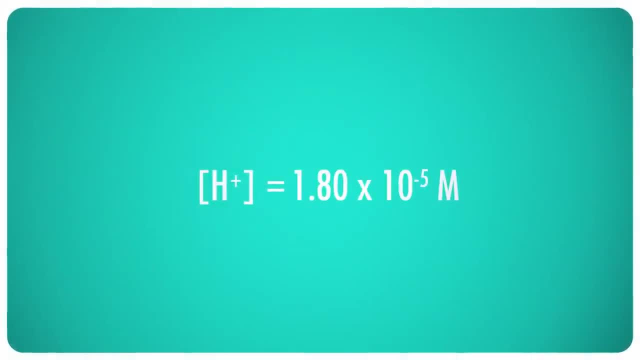 Well, pH is determined from the concentration of protons, which is in our equilibrium equation, so let's just solve for that. When you plug in the new acetic acid and acetate concentrations and the Ka, you get 1.80 times. 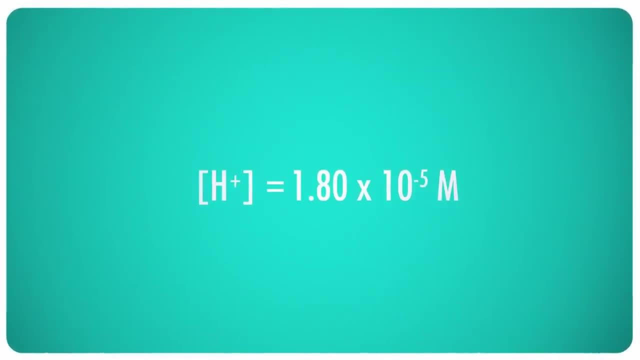 10 to the negative 5 moles per liter for the proton concentration, which translates to a pH of 4.746.. This is obviously not a big change from 4.746.. It's not a big change from 4.746.. 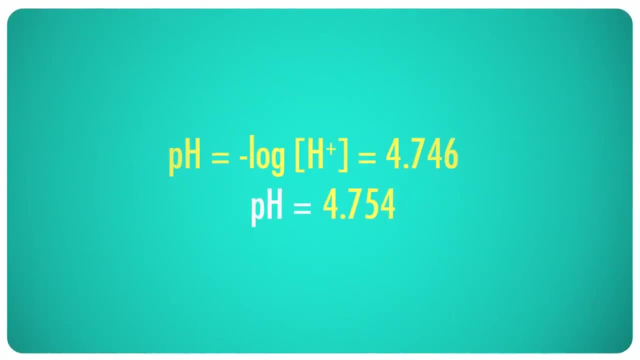 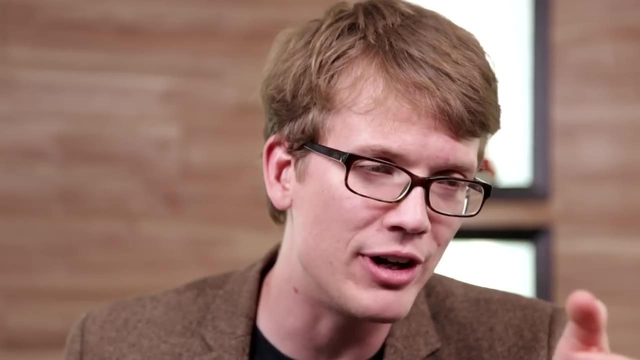 It's not a big change from 4.746.. In fact I had to go out to the fourth digit to see the pH change, which isn't even justified if you watch Crash Course Chemistry on Significant Figures. but I have to confess vinegar and 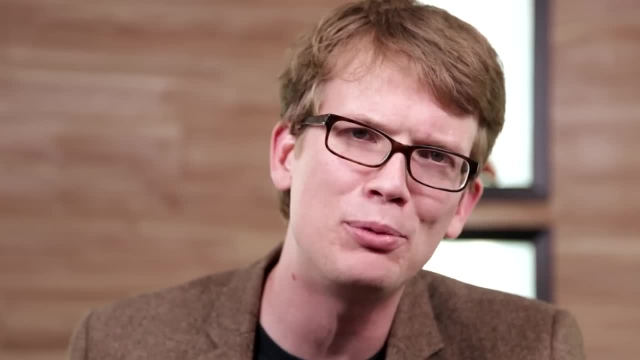 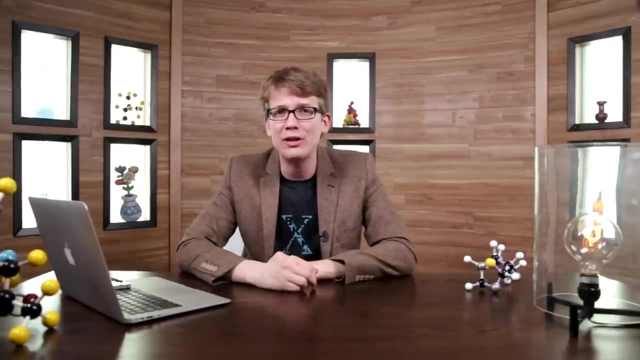 hydrochloric acid. they may make things easier to understand, but they're not exactly super relevant in terms of practical chemistry. Instead, I want you to see how this works in the real, real world. so let's consider the buffering system of the Clark Fork River. 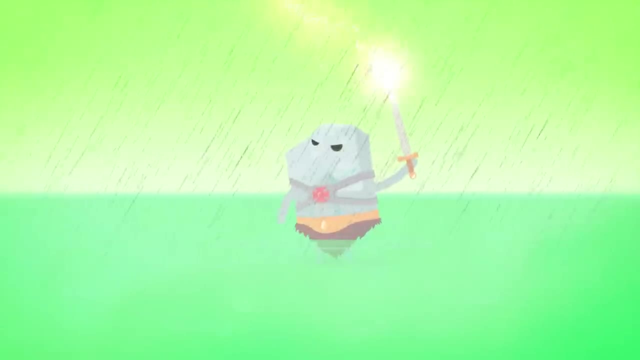 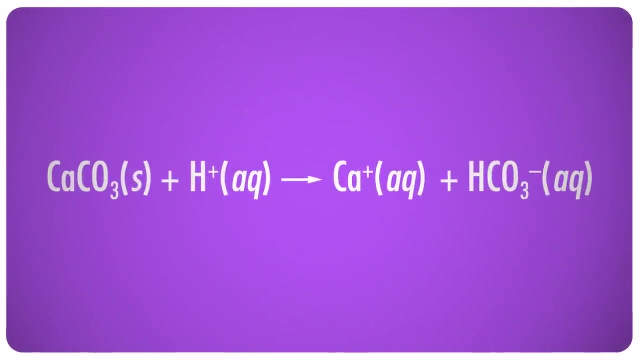 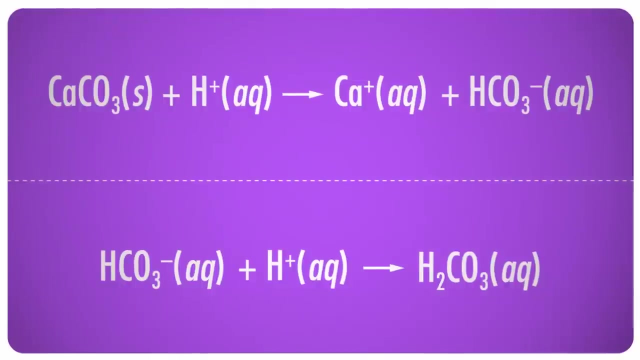 There, the reaction between dissolved limestone and acid rain really happens in three steps. First, the solid calcium carbonate reacts with the protons from acidic rain to form calcium and bicarbonate ions. The bicarbonate ions each have one hydrogen. As long as protons are available, the bicarbonate ions can grab a second proton to become uncharged. 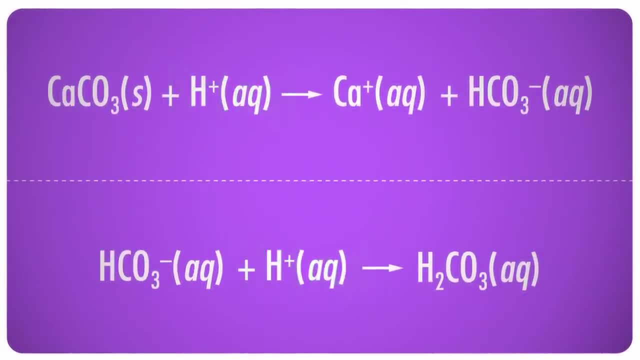 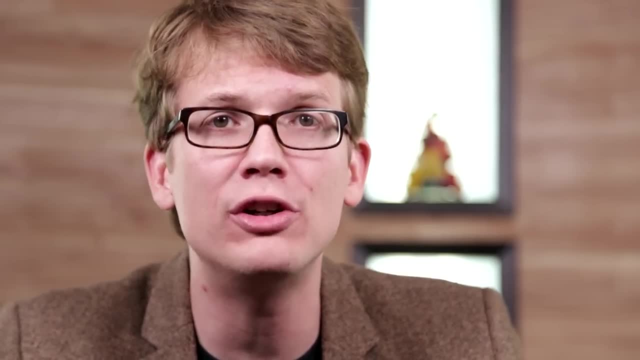 carbonic acid. As you can see, this chain reaction uses up two protons per molecule of calcium carbonate. That makes this process doubly powerful and that explains why the Clark Fork River is so resistant to acidification. But of course, buffers are not invincible. 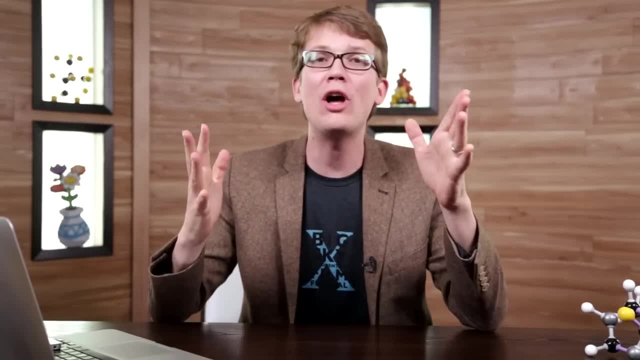 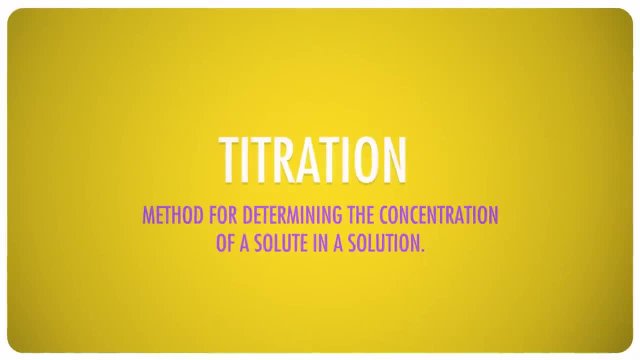 Add enough acid or base and even the best buffered solution will get overwhelmed. We call that threshold the buffering curve. It's the buffering capacity of the solution And we determine it in the lab using pH indicators through a process called titration. Earlier I used a pH indicator that showed an acidic pH by turning pink. 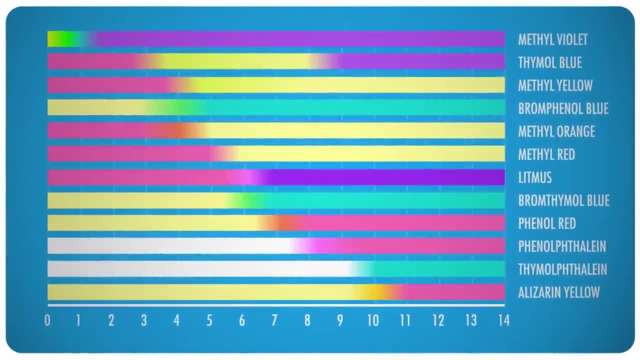 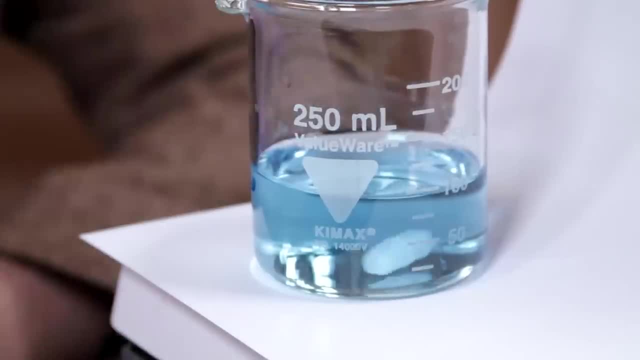 But there are lots of other indicators, each with different colors and a different pH. where it changes, This is called the indicator's endpoint. Here we have 100 milliliters of water from the river to which I've added some pH indicator. 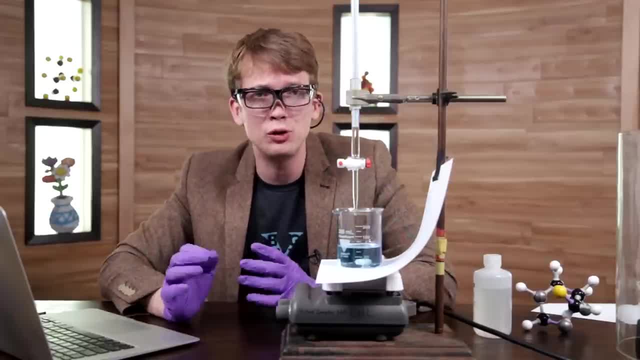 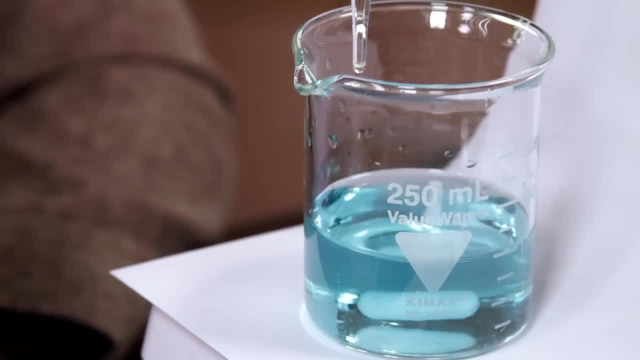 It's actually a mix of two different pH indicators, bromocresyl green and methyl red, that work together well for this reaction. It'll stay bluish in color for as long as the bicarbonate ions are around to keep the pH buffered above the indicator's endpoint of pH 4.. 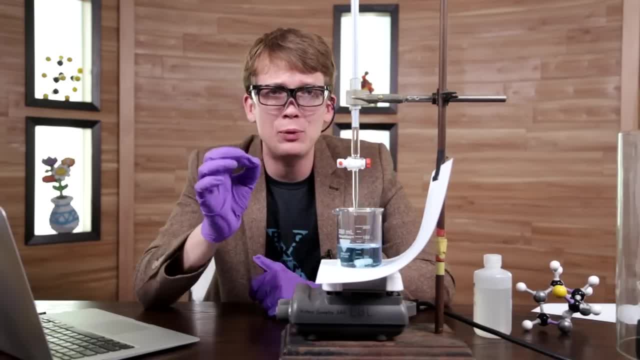 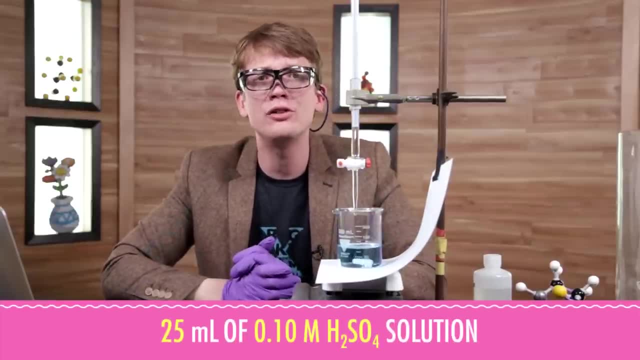 This long glass thing here is a burette. It's for dispensing liquids in a very controlled way, while also keeping track of how much you've dispensed At the moment. it contains exactly 25 milliliters of a 0.10 molar sulfuric acid solution. 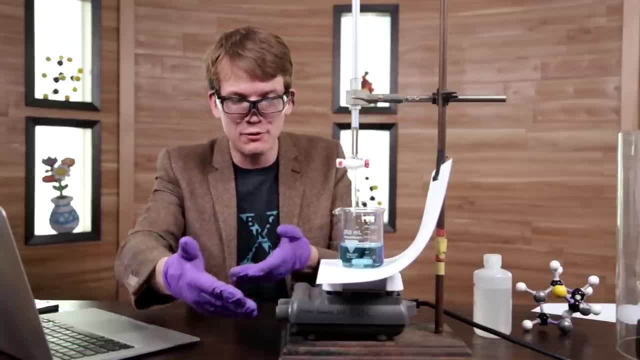 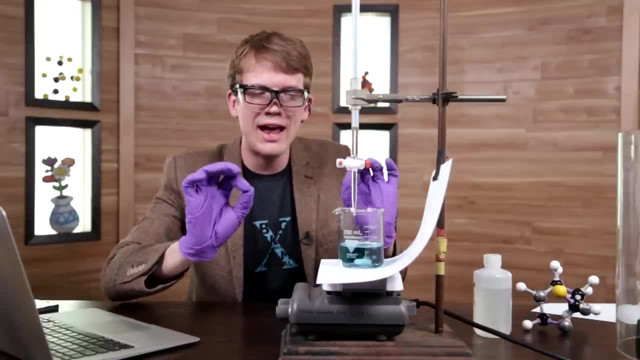 The thing to do is to add the acid very slowly, stirring as I go, which is being done for me by this automatic stir-y thing. You can do it a few ways. If you have a guess at how much you can put in, you can just sort of turn it on and let. 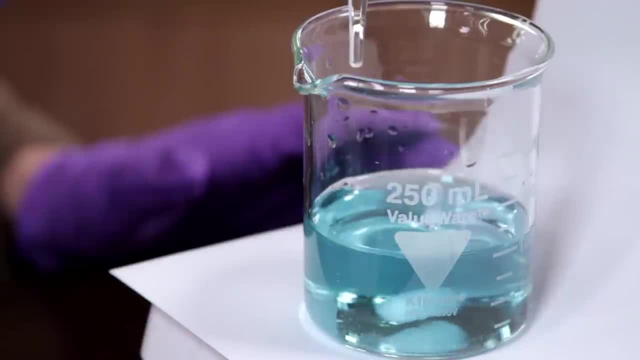 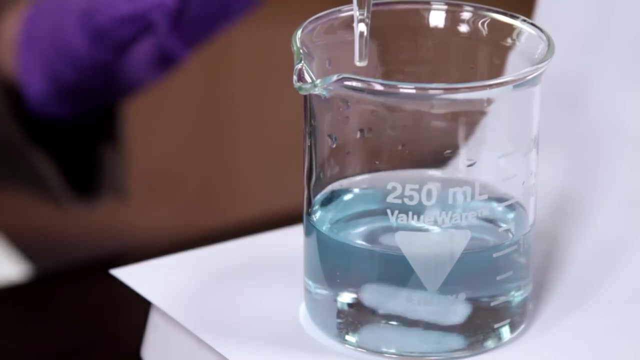 it go, But I don't know, so I'm just going to let it drip very slowly. You can turn it very slightly and you can actually get it to sort of do drippy drips. Then you're waiting to see if there's some changing happening, and there's a little bit. 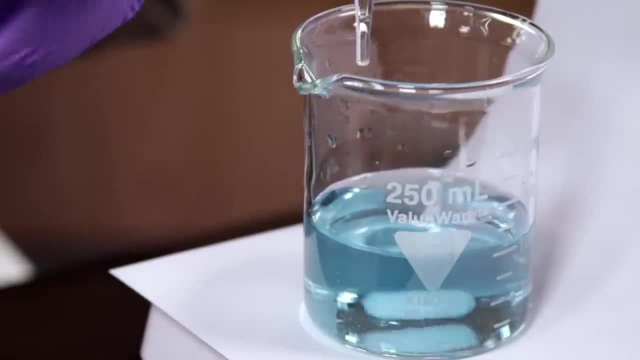 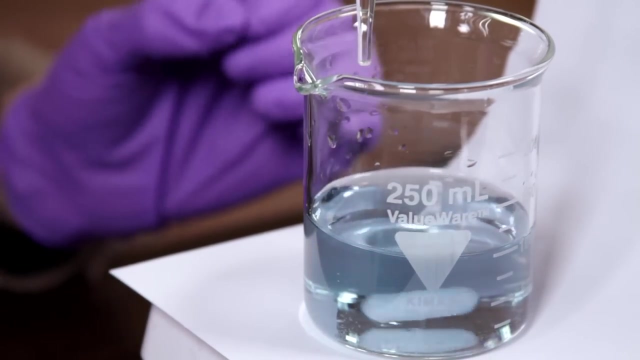 of changing happening, but now it's going back. We're getting closer And what I'm doing right now is I'm actually adding less than a drop at a time by going quickly past the opening in this little burette thing. I can actually see the reaction happening right before my eyes. 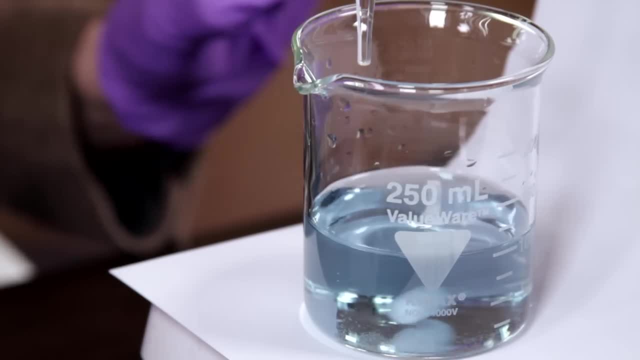 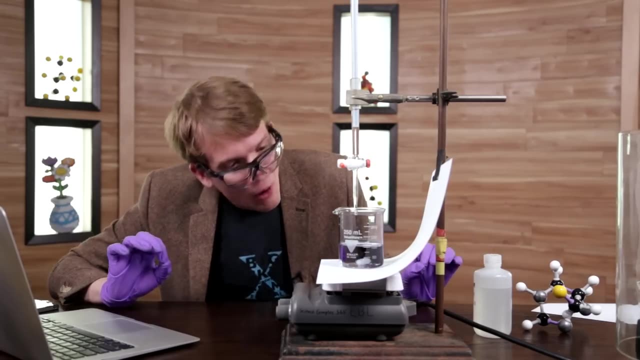 It's beautiful and then it goes back. It's right now a paler blue than it was before, which is exciting. That means we're getting very close. This is the stuff I get excited about. I know I'm a nerd. 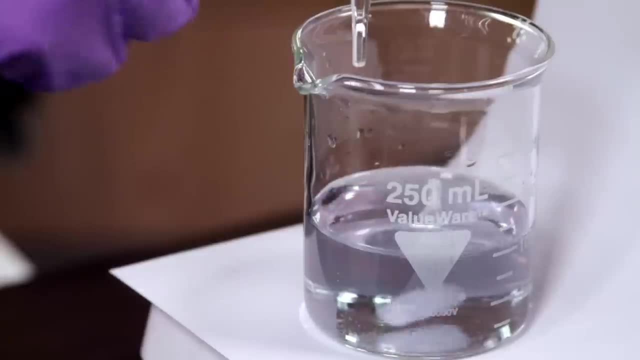 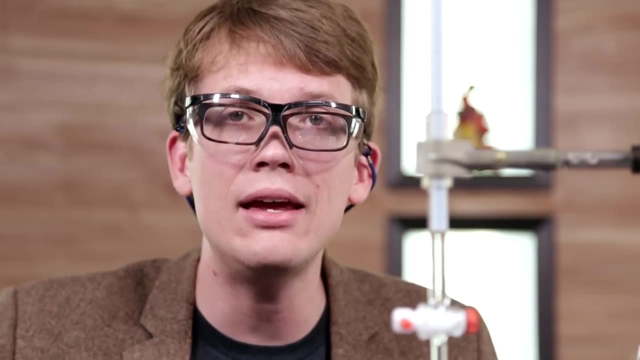 It's almost white. right now It's like pinkish, It's purpley. Oh beautiful, That was perfect. The solution is now staying pink, which means that I've exhausted its buffering capacity and the pH has dropped below the indicator's end point. 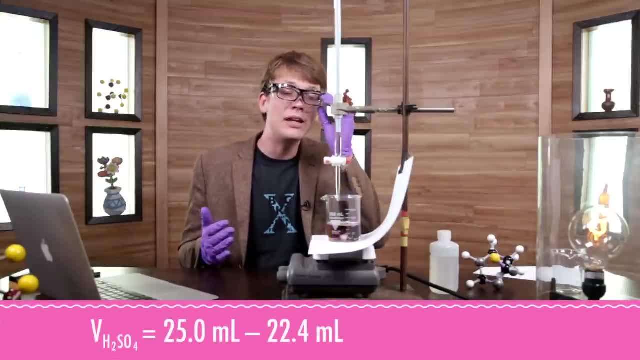 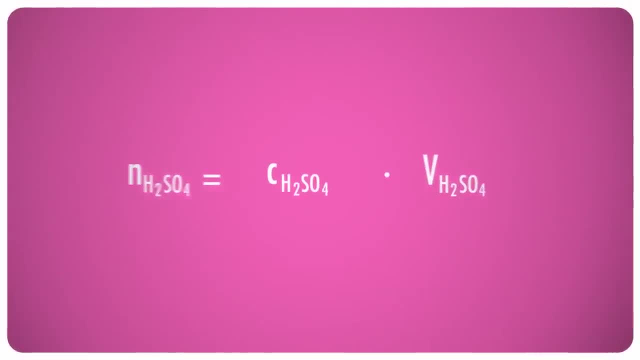 The volume in the pipette is now 22.4 milliliters, meaning that I used 2.6 milliliters, or 0.0026 liter of the acid solution. The acid solution is 0.1 molar, so multiplying these numbers together tells me that I used. 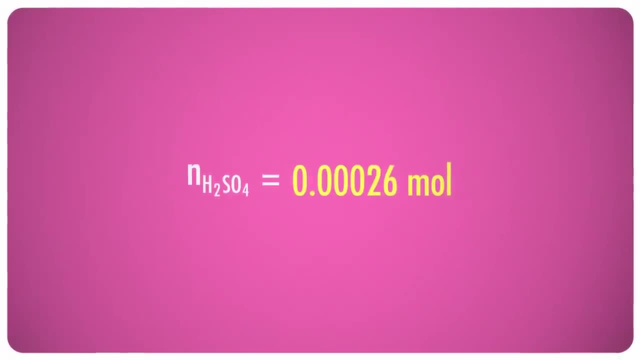 0.00026 molar. That's a whole lot more than a mole of H2SO4.. Sulfuric acid reacts in a 1 to 1 ratio with calcium carbonate, so assuming that calcium carbonate is the only buffer in the water, the 100 milliliters of river water here must 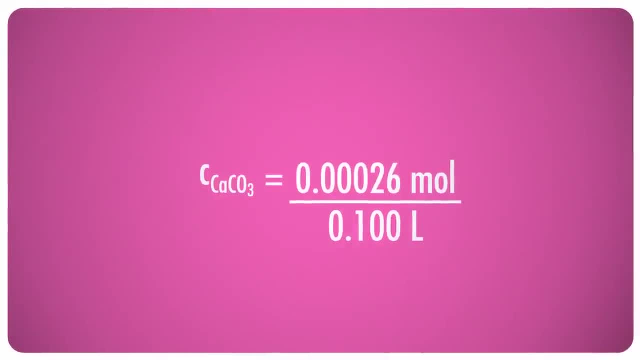 also contain 0.00026 moles of calcium carbonate, making it a 0.0026 molar or 2.6 millimolar solution. I'm a big fan of protecting the environment, but sometimes it is amazing to see what nature 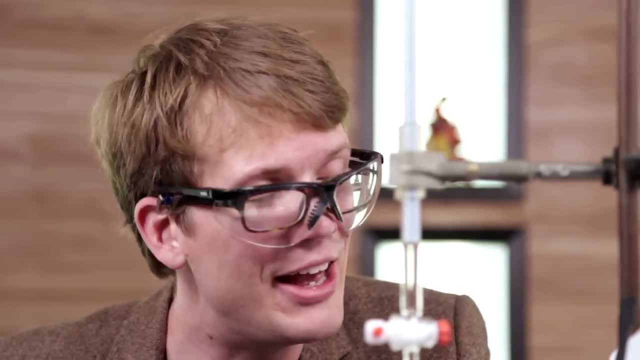 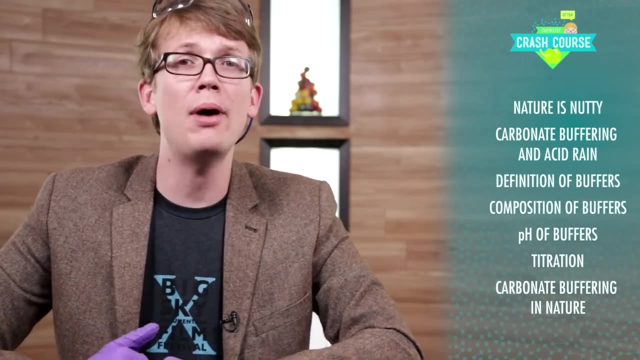 can do to protect itself. We live in an amazing world and I wouldn't trade it for anything, Not even Mars. Thanks for watching this episode of Crash Course Chemistry. If you were listening, you learned that some bodies of water like the Clark Fork River. 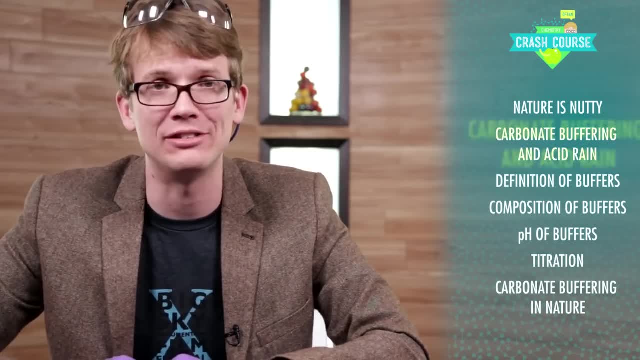 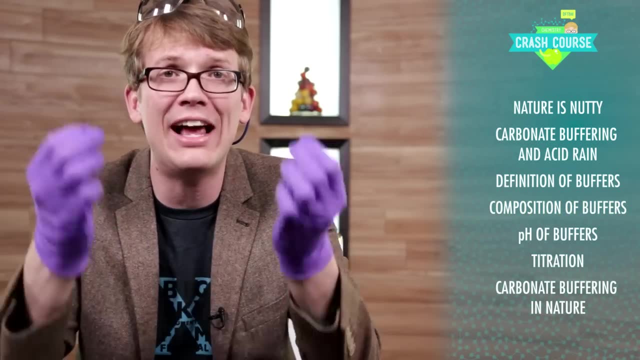 have natural protection from acid rain in the form of a buffering system. You learned that a buffer is a solution that resists changes in pH. You learned how to make a buffer solution, and you learned how to calculate the pH of such a solution by various methods, including titration. 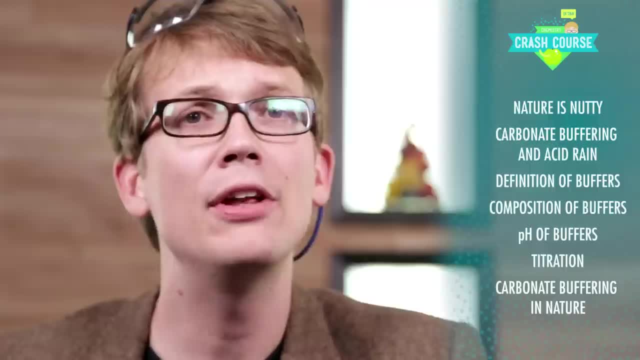 And, lastly, you learned the importance of the carbonate buffering system in nature. This episode was written by Kim Krieger and Edie Gonzalez, It was edited by Blake DePastino And the chemistry consultant was Dr Heiko Langner. 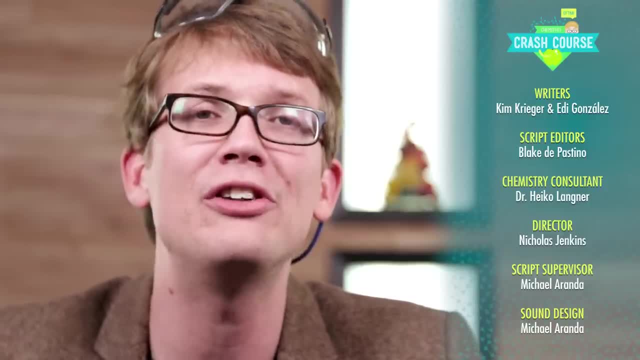 It was filmed, edited and directed by Nicholas Jenkins, Our script supervisor and sound designer was Michael Aranda, And our graphics team was Thought Cafe.